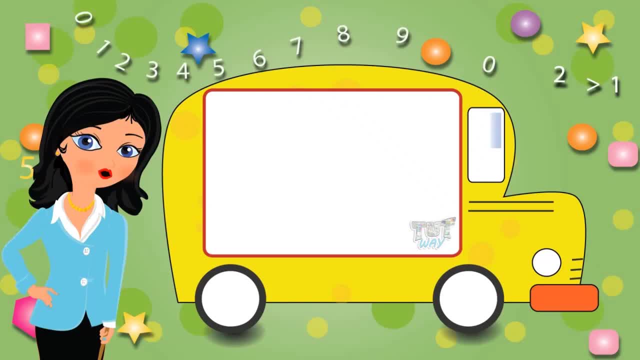 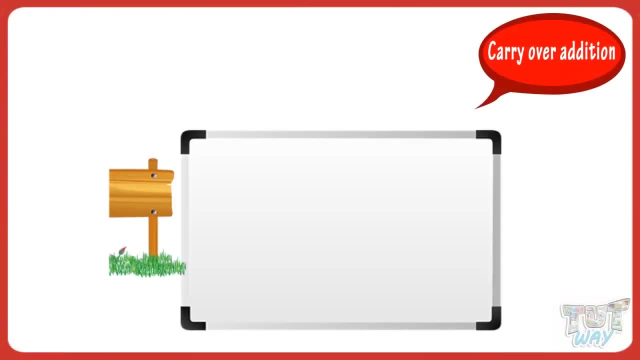 Hi kids, Today we will learn carryover addition. Before we start, we will revise a few questions on simple addition. First, add the ones place digits. 2 plus 2 equals 4.. Write the sum below ones place digits. Now add the tens place digits. 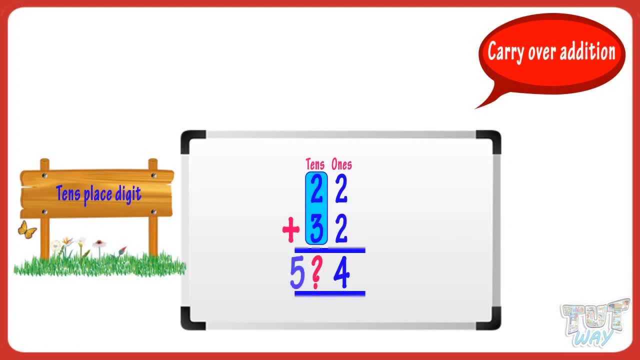 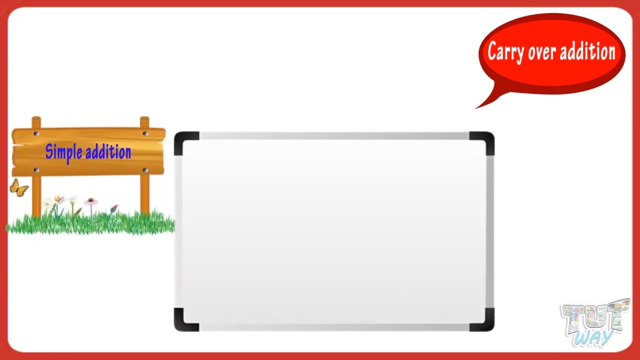 and write the sum right there below the tens place digits. Good, So we get: 22 plus 32 equals 52.. Here is another example. First of all add the ones place digits and write the sum below ones place digits. Now add the tens place digits and write the sum below tens place. 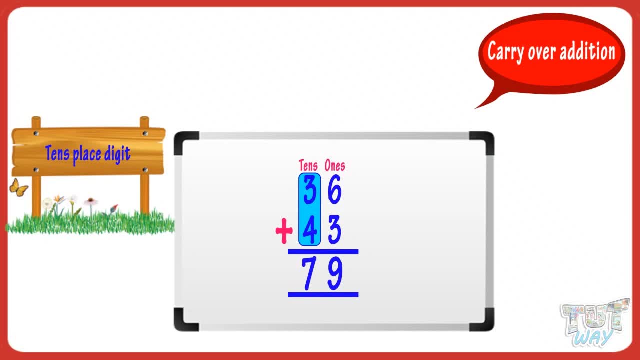 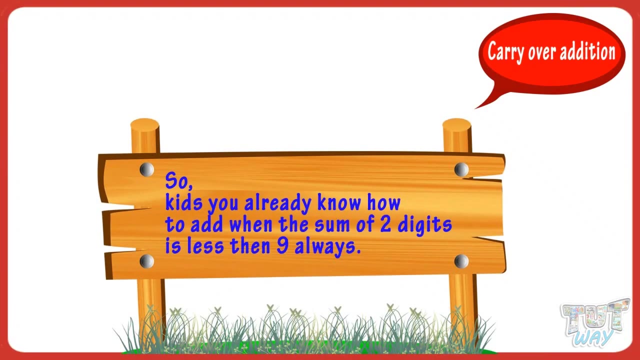 digits. Good, We get 22 plus 2 equals 4.. We get 36 plus 43 equals 79. So, kids, you already know how to add When the sum of two digits is less than nine, always. Now we will learn more on addition, So let's. 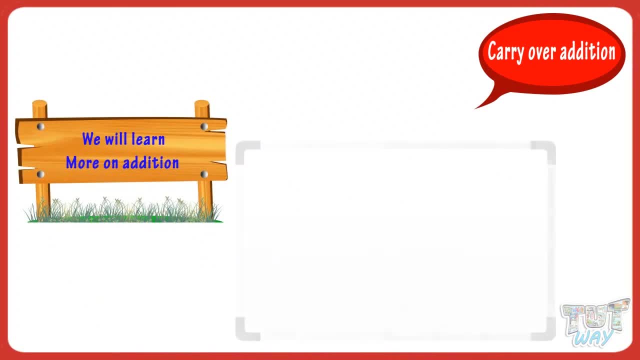 get started. First of all, we add the digits in ones place. So add 7 and 3.. Adding 7 and 3, we get 10.. Now 10 is a two digit number. So how to write 10? Write the digit in ones place, That's. 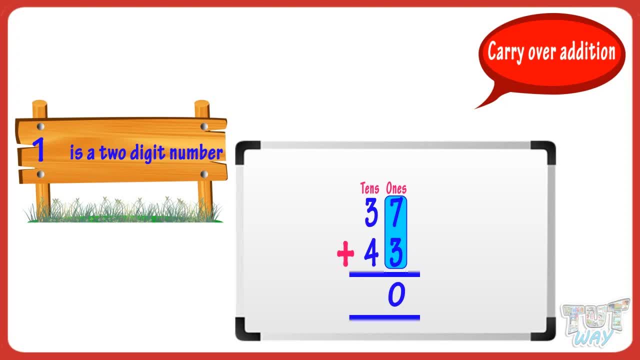 1,, 2,, 3,, 4,, 5,, 6,, 7,, 8,, 9,, 10.. That is zero below the ones. place digits in sum And carry over the tens digit and write it above the tens digit Like this. Now add the three digit. 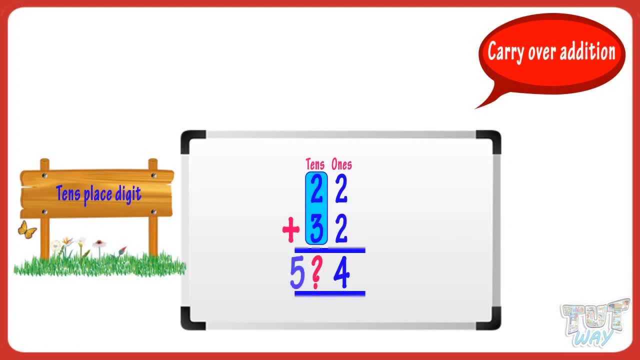 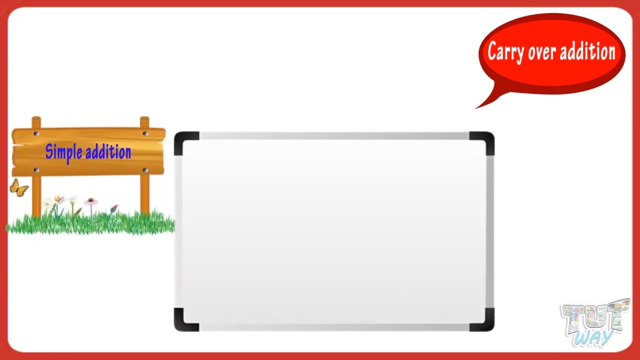 and write the sum right there below the tens place digits. Good, So we get: 22 plus 32 equals 52.. Here is another example. First of all add the ones place digits and write the sum below ones place digits. Now add the tens place digits and write the sum below tens place. 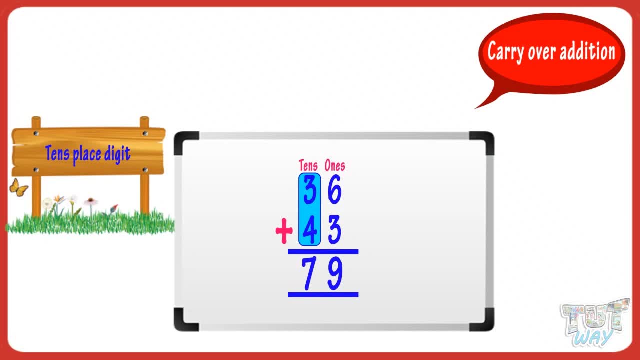 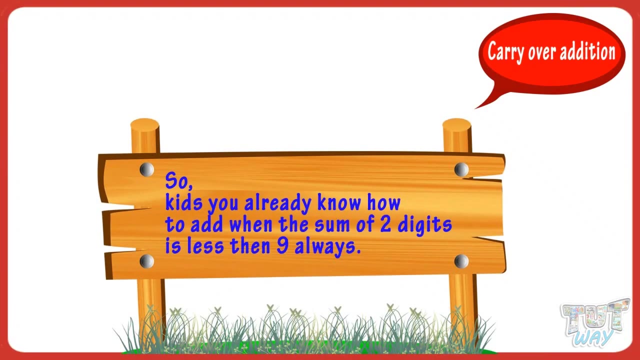 digits. Good, We get 22 plus 2 equals 4.. We get 36 plus 43 equals 79. So, kids, you already know how to add When the sum of two digits is less than nine, always. Now we will learn more on addition, So let's. 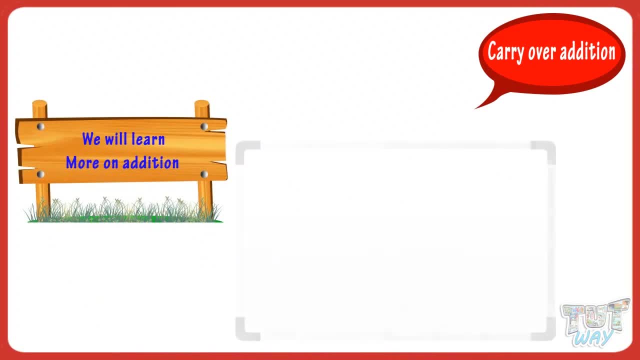 get started. First of all, we add the digits in ones place. So add 7 and 3.. Adding 7 and 3, we get 10.. Now 10 is a two digit number. So how to write 10? Write the digit in ones place, That's. 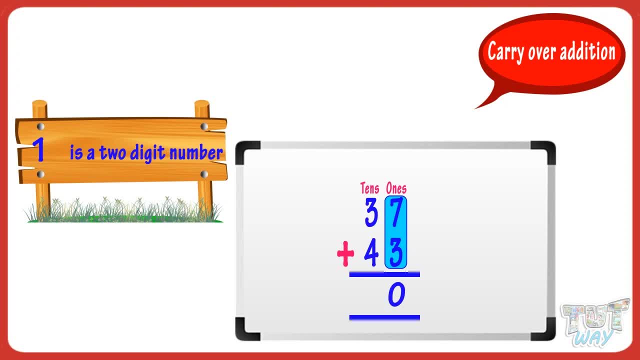 0 below the ones place digits in sum And carry over the tens digit and write it above the tens digit Like this: Now add the three digit in ten places, That is, 1,, 3 and 4.. 1 plus 3 plus 4.. 1 plus 3 equals 4. And 4 plus 4 equals 8.. Now write the sum of tens. 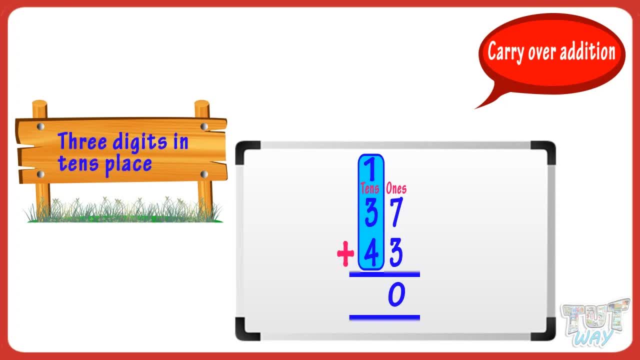 in ten places. That is, 1,, 3, and 4.. 1 plus 3 plus 4.. 1 plus 3 equals 4. And 4 plus 4 equals 8.. Now write the sum of tens digit below ten digits. Good, We got it. 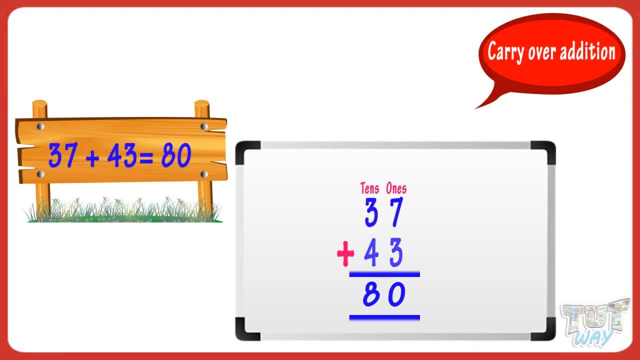 37 plus 43 equals 80.. Now let's do some more sums for practice, As, first of all, we add the digits in ones place. So add 7 and 5.. Adding 7 and 5, we get 12.. Now how to write. 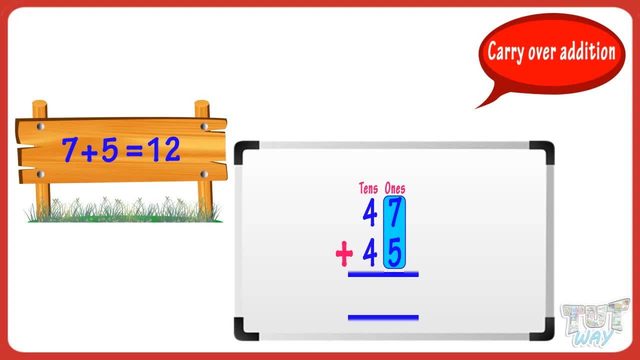 the digit in ones place. That's 1,, 3,, 4,, 5,, 6,, 7,, 8,, 9,, 10.. That is 12.. So add 7 and 4.. Now let's do some more sums for practice. Here we go. Write the digit in ones place. That's 1, 3,, 4,, 5,, 6,, 7,, 8,, 9, 10.. That's 1, 3, 4, 5, 6,. 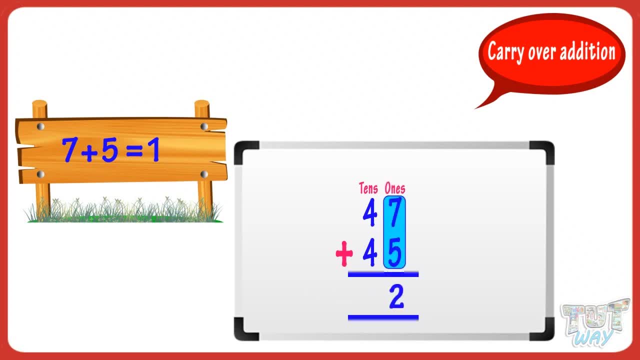 7,, 8,, 9, 10.. That's 1,, 3,, 4,, 5,, 6,, 7,, 8, 10.. Now how to write the digits in ones place Below the ones place digits And carry over the tens digit And write it above the tens. 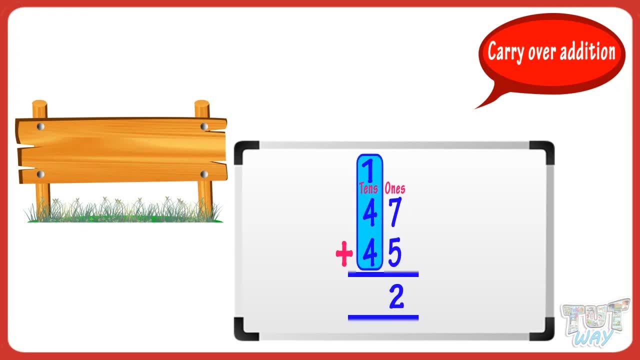 digits Like this: Now add the 3 digits in tens place: 1,, 3,, 4,, 5,, 6,, 7,, 8,, 9,, 10,, 11,. Now add the three digits in tens place. 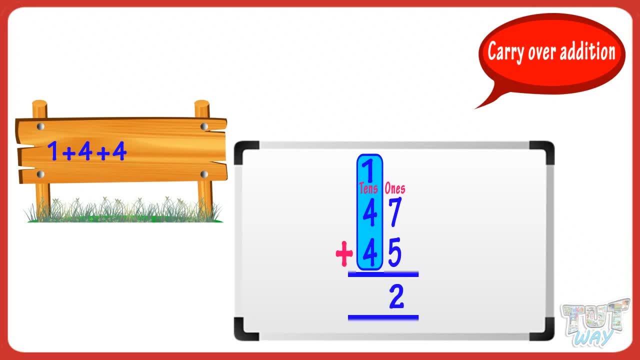 One plus four plus four. One plus four equals five. Five plus four equals nine. Now write the sum of tens digits below tens digits. Good, We got it. Forty-seven plus forty-five equals ninety. Let's do some more sums for practice. 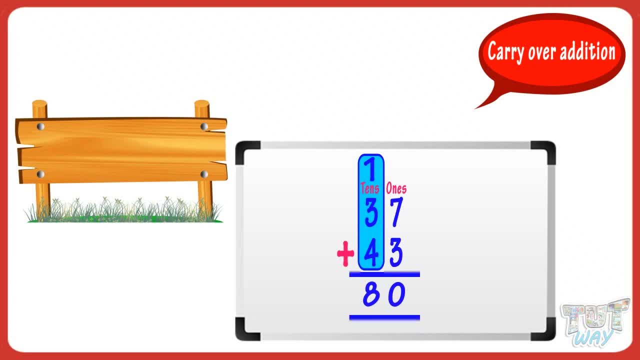 digit below ten digits. Good, We got it. 37 plus 43 equals 80.. Now let's do some more sums for practice, As first of all we add the digits in ones place. So add 7 and 5.. Adding 7 and 5, we get 12.. Now how to write 12?? Write the. 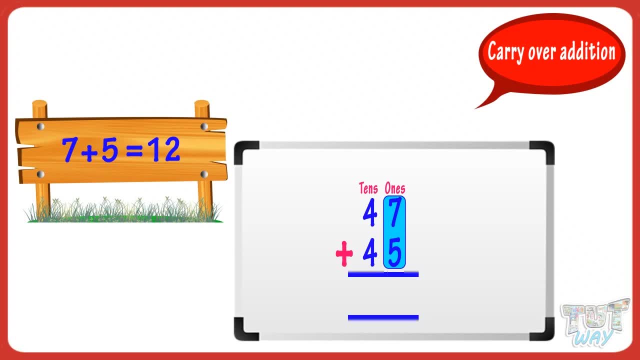 digit in ones place, That is, 2 below the ones place digits, And carry over the tens digit And write it above the tens digit crack String by pressing X like this: Now add the three digits in tens place: 1 plus 4 plus 4.. 2 plus 4 plus 5,. 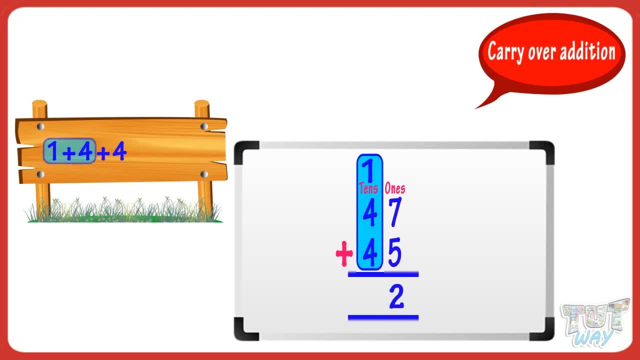 want see. now write it above the 10s digits Like this: 1 plus 4 plus 4 equals 5.. Now write the 1 and right them below tens digits. Add 3 together and write above the tens digits like this: 1 plus 4 plus 4 will write 10 in place level. 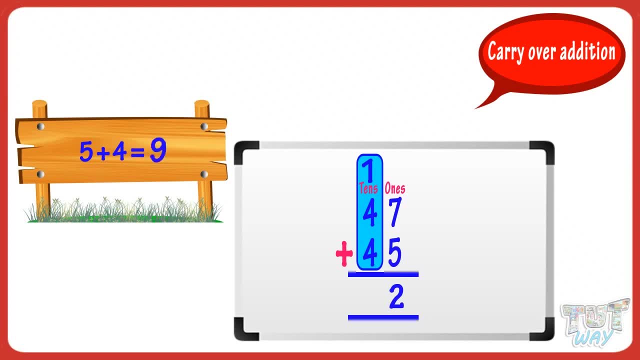 1 plus 4 plus 4 will write 4.. Now write the 2 and 1 will write a surmise using במ� to write it above the tens and 10s digits like this: Now add the three digits in tens places: 1 plus. 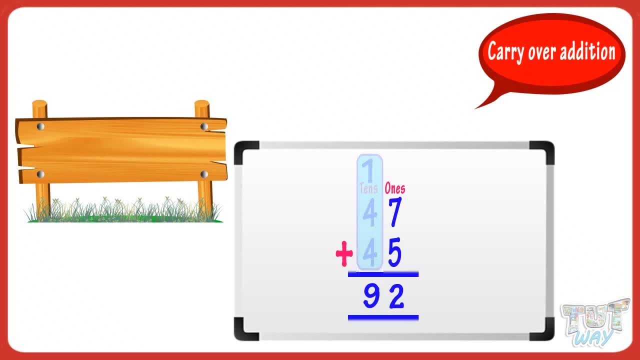 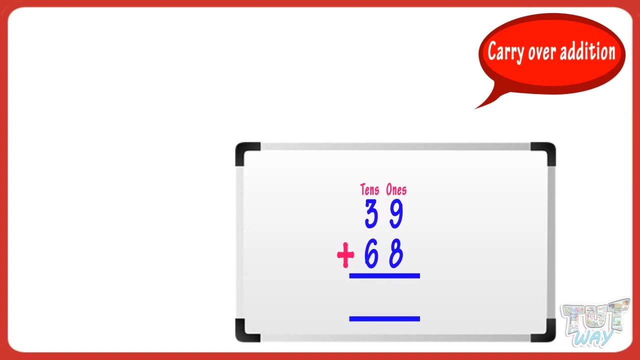 sum of tens digits below tens digits. Good, We got it. 47 plus 45 equals 90.. Let's do some more sums for practice, As, first of all, we add the digits in ones place. so add 9 and 8.. Adding 9 and 8, we get 17.. Now how to write 17?? Write the digit in ones place. 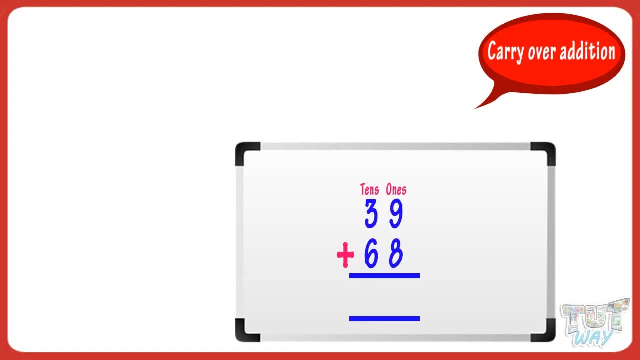 As first of all, we add the digits in ones place. so add nine and eight. Adding nine and eight, we get seventeen. Now how to write seventeen? Write the digit in ones place, that is seven below the ones place digits in sum: 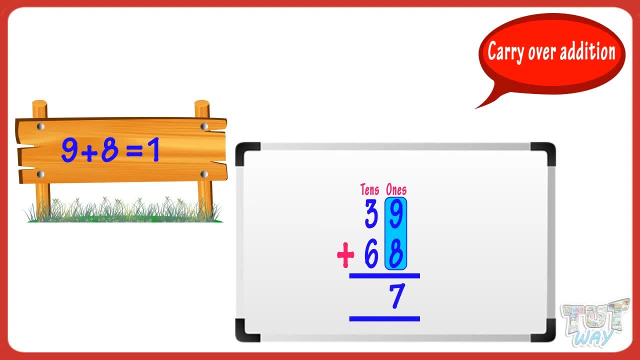 And carry over the tens digit and write it above the ten digits in sum like this: Good, Now add the three digits. Write the digits in tens place, that is one, three and six. One plus three equals four. Four plus six equals ten. 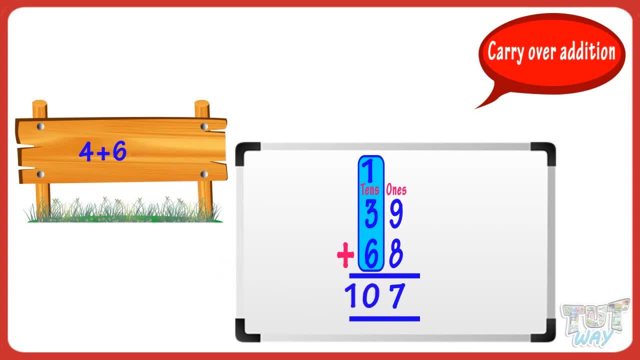 Now write the two digit sums like this: Good, We got it. Thirty-nine plus sixty-eight equals twenty. One plus five equals one hundred and seven. One plus five equals one hundred and seven. Good, Let's do some more sums for practice. 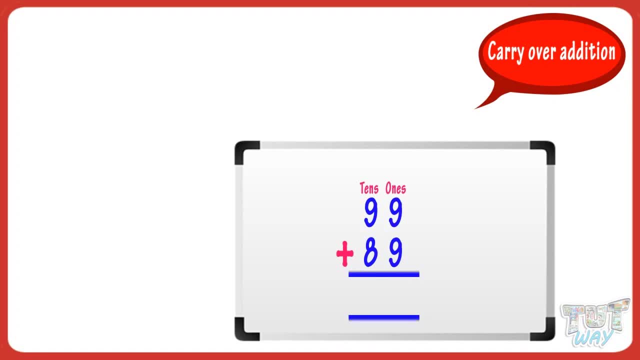 As first of all we add the digits in ones place. so add nine and nine, We get eighteen. Now how to write eighteen? Write the digit in ones place, that is seven, below the ones place digits in sum. Write the digit in ones place, that is one, three and six. 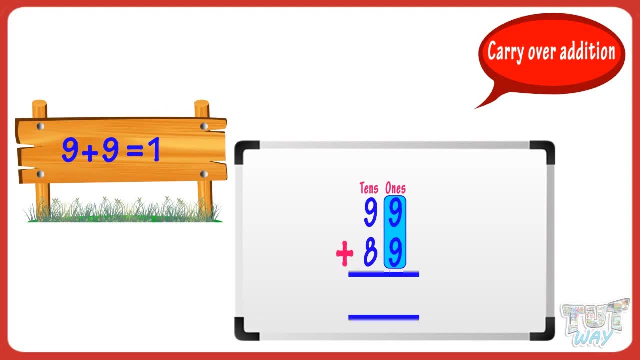 place that is 8 below the ones place digits in sum, and carry over the tens digit and write it above the tens digit in sum like this: Now add the three digits in tens place: 1 plus 9 plus 8.. one plus nine equals ten. Ten plus eight equals eighteen. Now write the two digit. 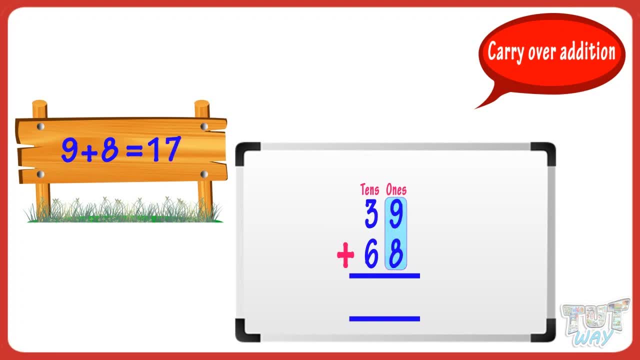 that is 7 below the ones place digits in sum, And carry over the tens digit and write it above the tens digits in sum, Like this. Good, Now add the three digits in tens place, that is, 1,, 3, and 6.. 1 plus. 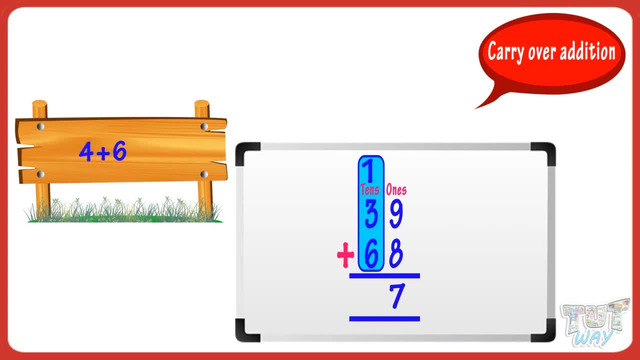 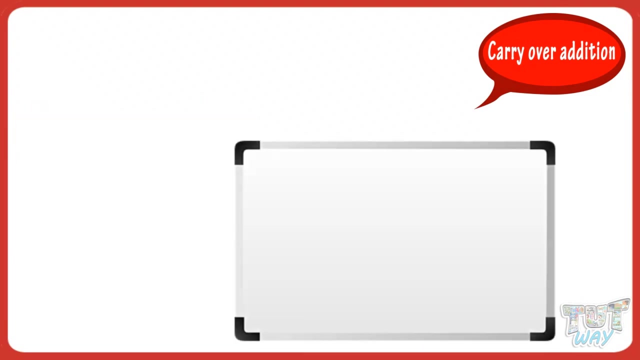 3 equals 4.. 4 plus 6 equals 10.. Now write the two digit sums like this: Good, We got it. 39 plus 68 equals 107.. Good, Let's do some more sums for practice, As first. 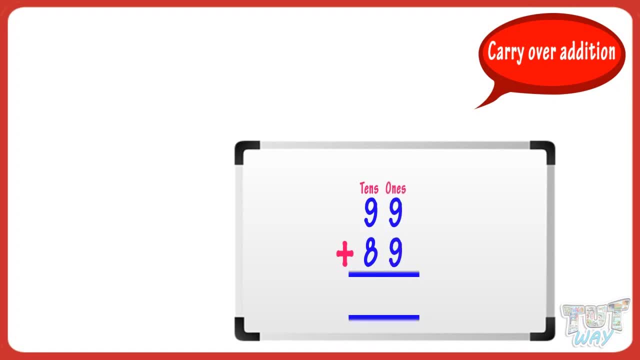 of all, we add the digits in ones place. so add 9 and 9. We get 18.. Now how to write 18? Write the digit in ones place that is 8 below the ones place digits in sum And carry over the tens digit and write it above the tens digit in sum, Like. 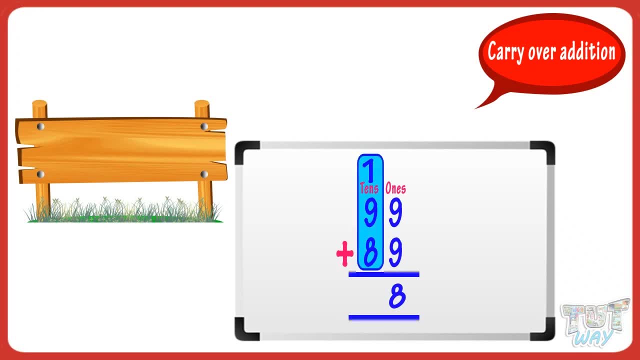 this: Now add the three digits in tens place, that is, 1,, 3, and 6.. 1 plus 6 equals 10.. And carry over the tens digit and write it above the tens digits in sum Like this: 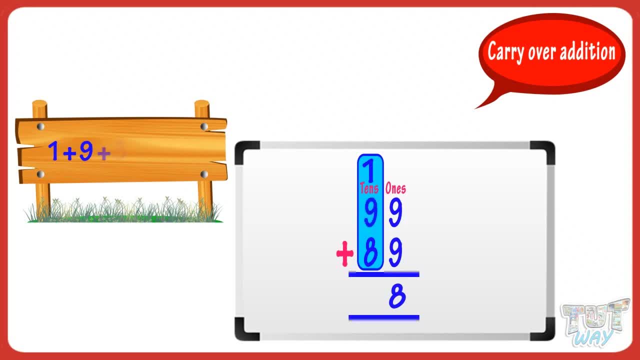 1 plus 9 equals 8.. 1 plus 9 equals 10.. 10 plus 8 equals 18.. Now write the two digit sums like this: Here 1 is written below hundreds place And 8 is written below tens.